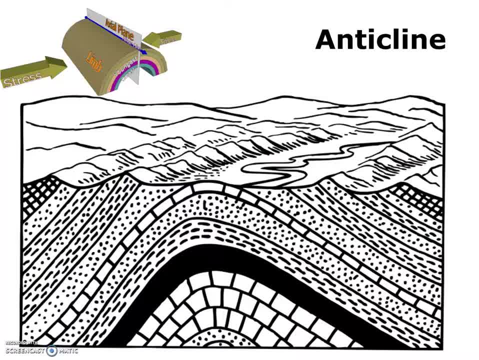 Take a quick look at the image of the anticline at the top of this slide. Do you notice that the axis of the fold is flat and horizontal? This is called a non- plunging fold because the fold axis is horizontal. When this is the case and the anticline experiences erosion, a particular outcrop pattern, 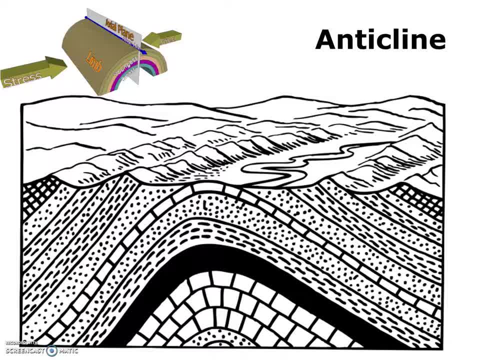 will occur on the surface of the earth. In the larger image, do you see that this is an anticlne as well? Notice that the top of it has also been eroded And we see exposure of the interior of the anticline. As the surface is eroded, this non-plunging fold is encrypted by the sources of this non-plunging fold. Of course, this is replacement. This is a personal idea, but perhaps I should mention it once again In this picture. imagine how tight the intert ihte climb was. carta s России. 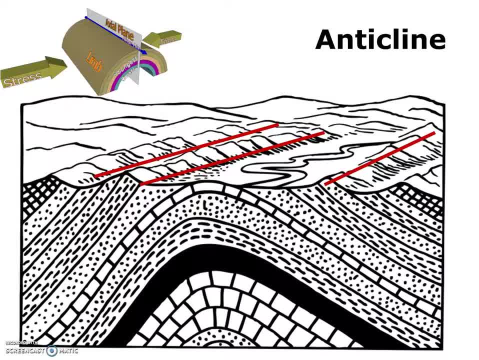 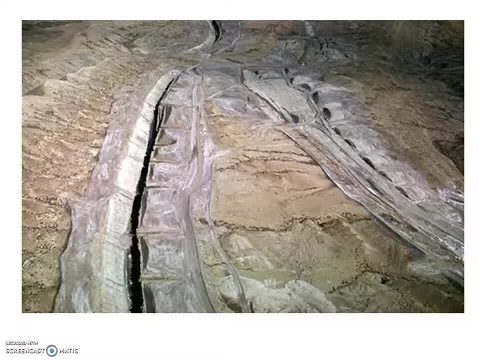 will form parallel outcrop patterns, as noted in the red lines. This is a picture of the Bentonite open-cut mine from the Cretaceous-Mowry formation, which is a small sincline in Sheep Mountain Wyoming. Notice the parallel outcrop pattern that 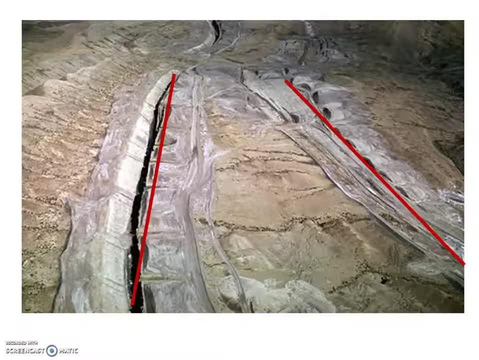 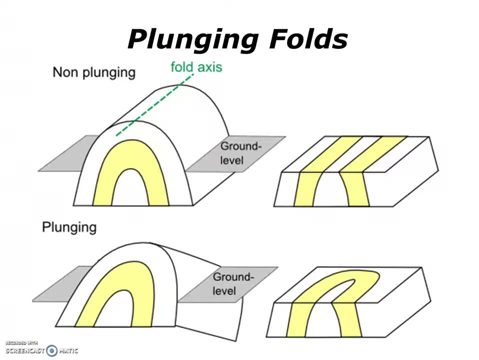 is formed as this non-plunging fold has been eroded. Not all folds are non-plunging. Note that the top fold on this image is non-plunging, like those that we've seen in previous slides. Do you see that the eroded surface will? 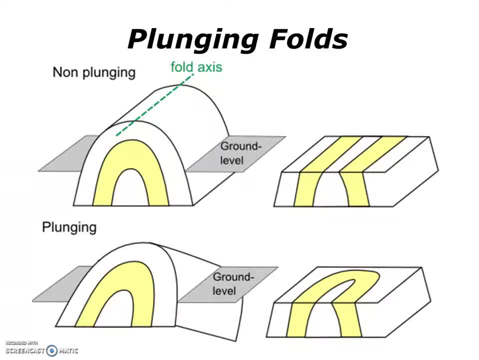 produce parallel outcrops. In the case of a plunging fold, as those seen on the bottom of this image, the fold axis is no longer horizontal As this type of fold is eroded. rather than parallel outcrops, the pattern we will see will be a: 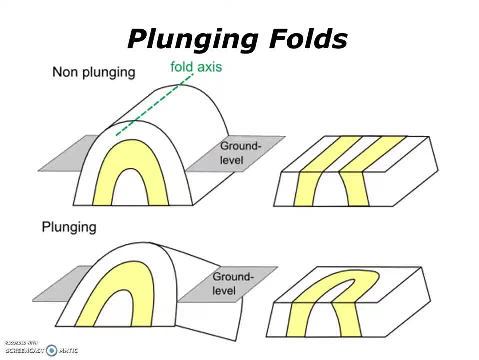 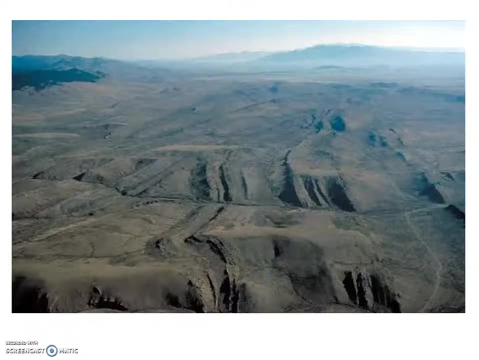 U-shape. In this case this is a plunging anticline, although sinclines can also be plunging and form similar outcrop patterns. Here in this image we see an eroded surface of the earth. Note the outcrop pattern. Would you expect this outcrop pattern to be a plunging or a? 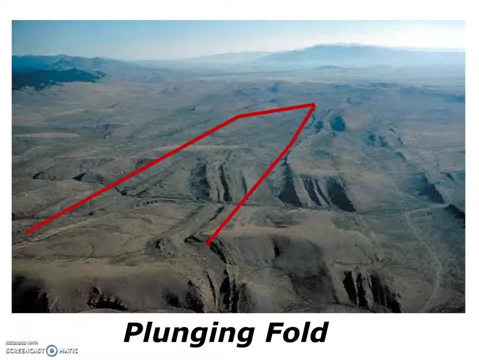 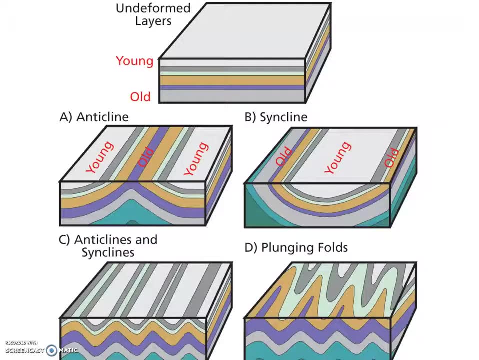 non-plunging fold. It's a plunging fold, as you can see by the U-shape outcrop pattern. We can also consider relative geologic age when looking at outcrops and trying to determine whether the outcrops are anticlines or sinclines. Note that in this block diagram that we see an. 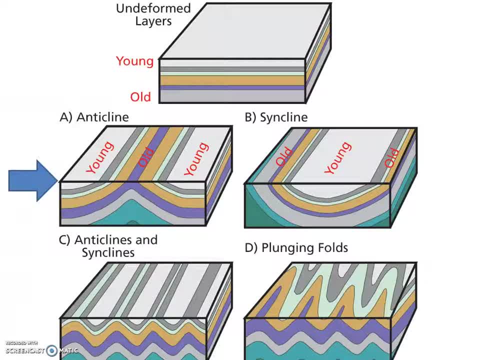 anticline. Younger rock layers of this anticline are found on the limbs of the fold, As we can see on the geologic map on the top of the block diagram. Also, note that this ooklid fold has an autocline. Also note that this ooklid fold has an autocline, as we can see on the geologic map on the top of the block diagram. 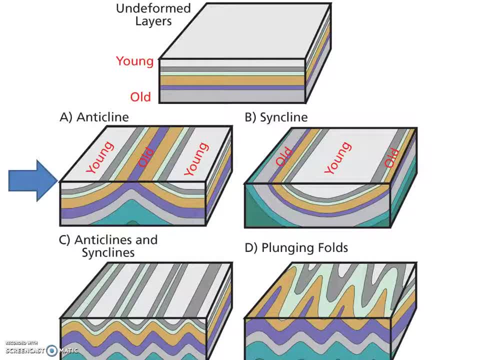 Also note that this oak side fold has an unclocked piece of the ous that blocks the outclined fold. the older rock layers are found along the axis of the fold. In the case of a syncline like this block diagram, it's the opposite. Notice that the older rock 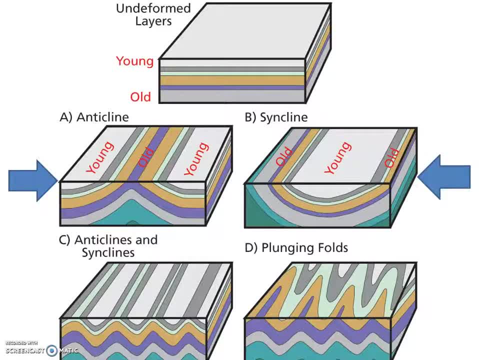 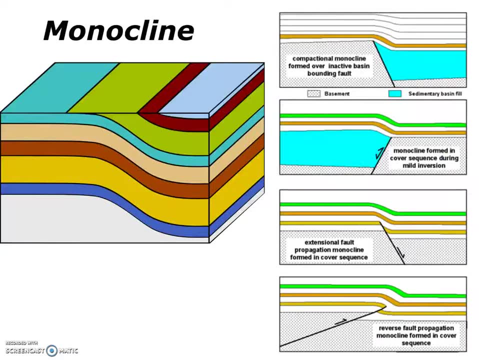 layers are found on the limbs of the fold, while the younger rock layers outcrop along the axis on the geologic map on the top. Another type of fold that can form in areas of compression is known as a monocline. Monoclines form as 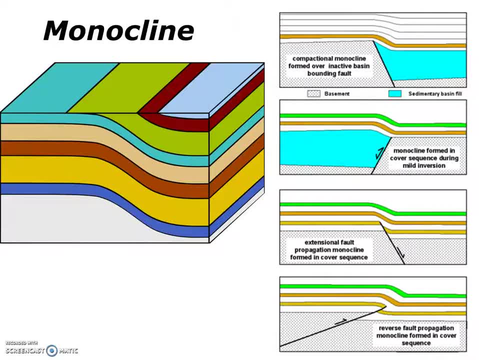 large step-like folds and otherwise horizontal sedimentary strata, and they only have one limb. Monoclines are often the product of a reverse fault that has occurred somewhere deep in the crest. Sometimes the sedimentary rocks above the fault can deform as a ductile solid folding over the fault to produce a 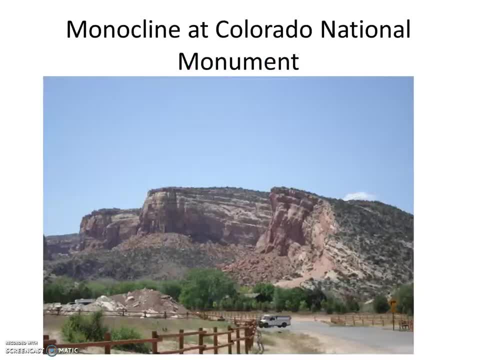 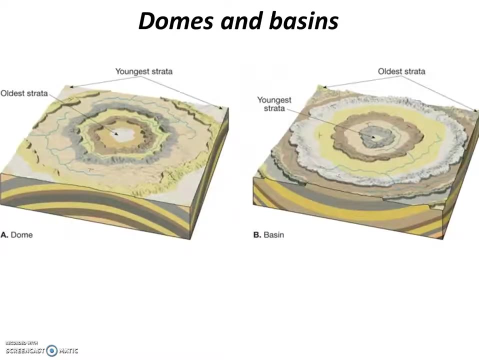 monocline. This is a picture of a well-known monoclinal fold present in western Colorado at the Colorado National Monument. Notice the dipping limb. Two other types of folds are domes and basins. Be careful not to confuse these with valleys and hilltops. It is often the case that 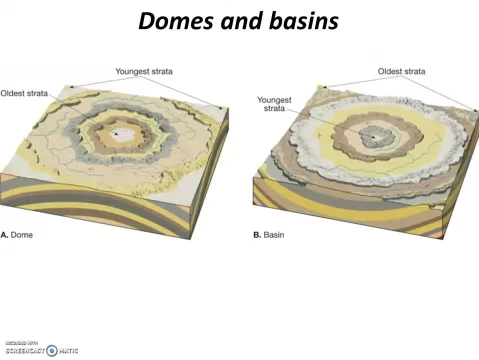 domes. structural domes and basins form different landforms on the surface, rather than valleys and hills. A structural dome like that seen on the left is an upward displacement of rocks. It forms a circular or slightly elongated outcrop.